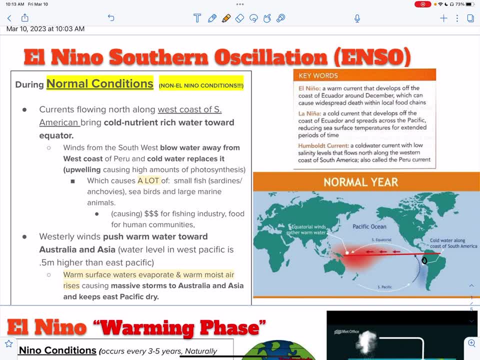 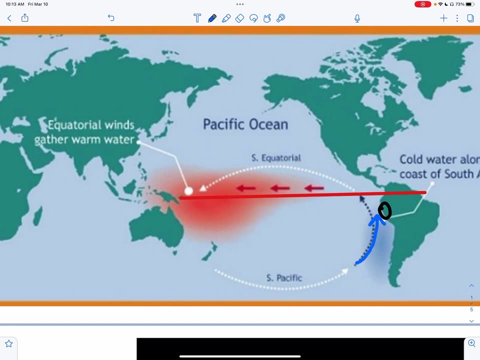 during normal conditions. A water current will be flowing during normal conditions, So that's going to be will flow north along the west coast of South America. it brings cold, nutrient rich water. this is your Humboldt current, so you have a current that will flow north. remember, if we have water coming from the deep, it's also going to be bringing along. 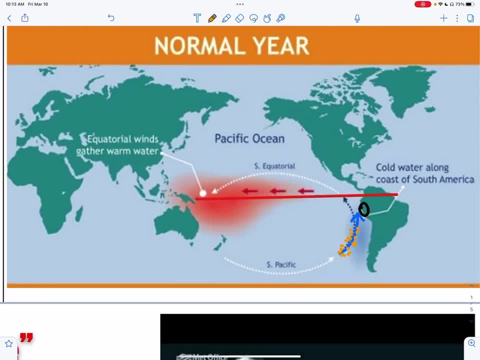 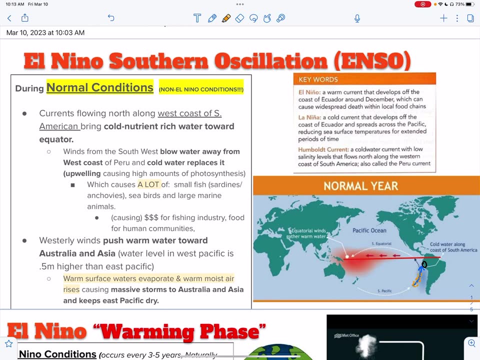 with it a lot of nutrients, which will be great for our producer population. okay, and so what's going to allow this current to be coming to the west coast of Peru? bring up all that nutrients? it's winds that blow southwest. they blow water away from the west coast, so these are. 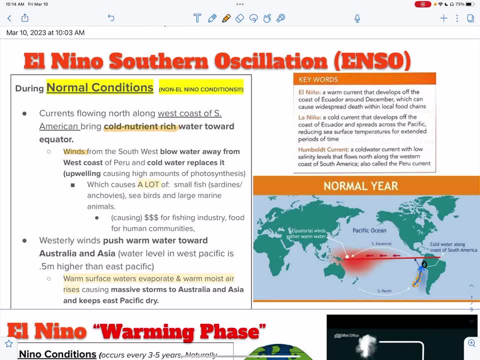 our trade winds just based on the trade route that was taken. that's why they're called trade winds- really strong trade winds that will blow water off the coast of Peru- and I shouldn't say really strong, they're just they're strong. so blow water away from the west coast of Peru. cold water will replace it, because that's going. 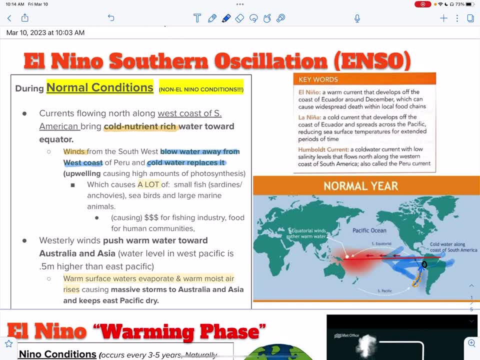 to be an offshore wind. it's moving a bunch of water and it causes low water pressure at the surface, just like we talked about on Monday, five days ago, and that low water pressure has to be replaced by water, and that water that replaces it is coming from. 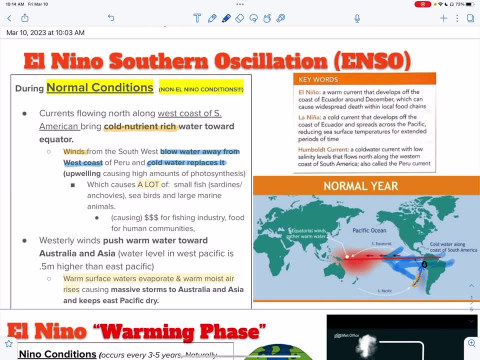 the deep, not only is water moving up, but also all the dissolved nutrients, and this is going to cause upwelling. and along with that upwelling we're going to have a lot of productivity, a lot of primary productivity, so a lot of photosynthesis happening quickly. if we have a lot of photosynthesis from 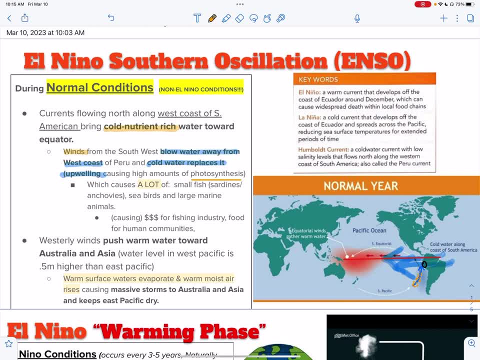 our producers, then we can assume we're going to have a lot of primary consumers. so small fish soup, plankton, sardines, anchovies- anchovies are brought up a lot in the exam questions- seabirds- they're to feed at the surface large marine animals, whales, sharks. the food chain follows each other. 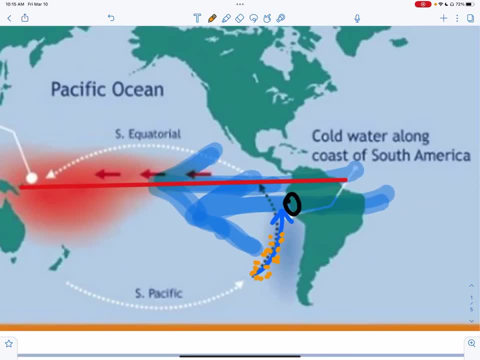 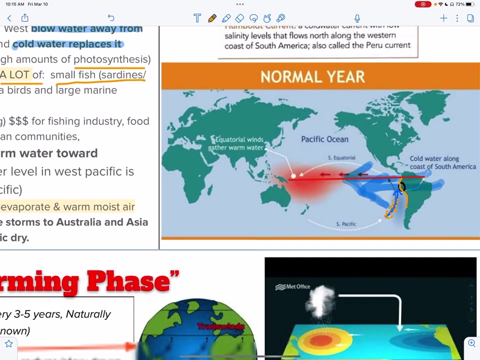 okay, if we consider the coast of Peru and we know like what kind of demographic of the country it is, it is not what we would consider a high-income country. so they're most likely going to people living on the coast there are going to be very heavily rely relying on their fish catches and 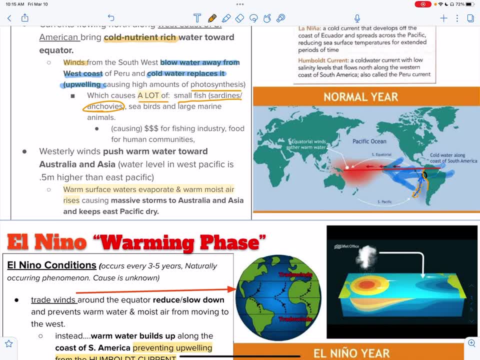 and what they do for fishing is a business, and so this allows them to maintain a lot of money for their fishing industry. it allows for food for their communities and jobs. okay, and just to touch on what's going to happen on the other side, then our trade winds. 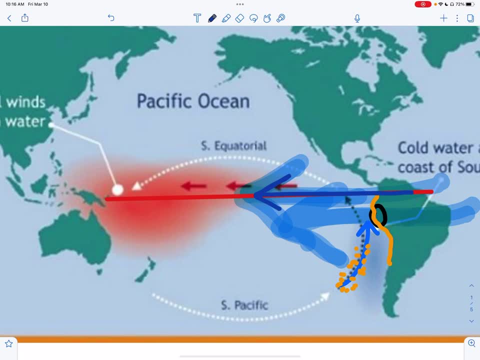 are relatively strong, they're normal. they're pushing all this warm water off the coast of Peru over to the Australasia area or Australia, Asia. that's good for them, because if we know what happens with warm water, especially when you have warm air blowing over it, it happens here all the time in the summer you're going to have evaporation. 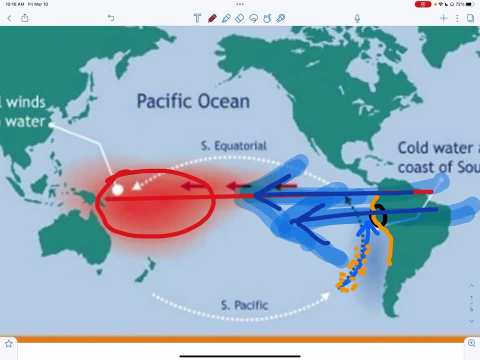 I shouldn't have made those arrows blue. maybe I have a lot of evaporation, which will then cause a lot of condensation, and what's going to come with that then is precipitation. that's good, because Australia has a lot of fires often. things to consider within the ocean, though, is that when we have 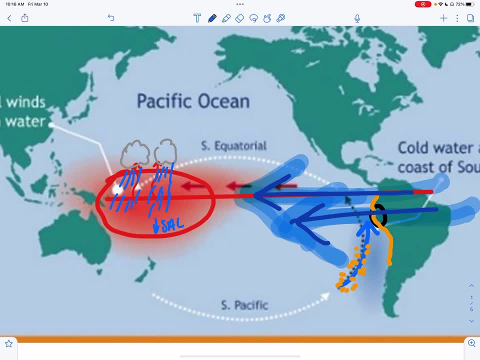 a lot of precipitation, we're going to decrease salinity. when you have a lot of cloud cover, cloud cover is actually going to decrease the sun penetration into the water, which will decrease photosynthesis a bit. photosynthesizers need sunlight so they can synthesize glucose. 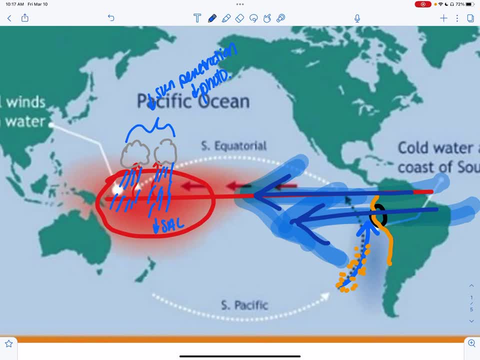 and not only that: when we have winds, we or clouds, we need to consider that there's going to be storms, there probably a lot of wind that's going to stir up a lot of your water. it's going to produce a lot of waves. waves are produced by wind and cause the water be pretty turbid, which in and 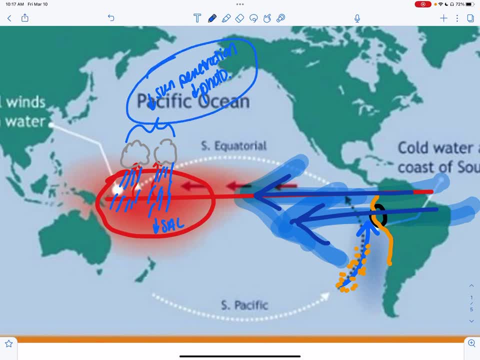 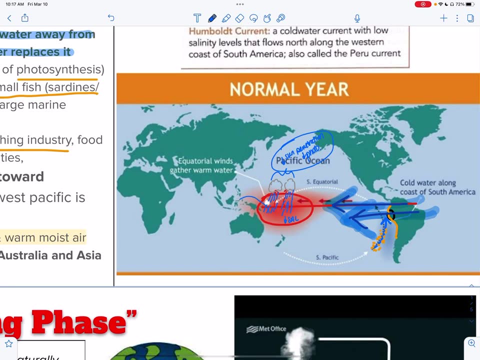 of itself will then again block sunlight penetration and decrease the rate of photosynthesis. not that these exam questions focus on the Australasia area, the Australian Asia area. they do focus on this happening in Peru, and we will have similar types of effects from lower sunlight penetration off the coast of Peru during an El Nino, but again, 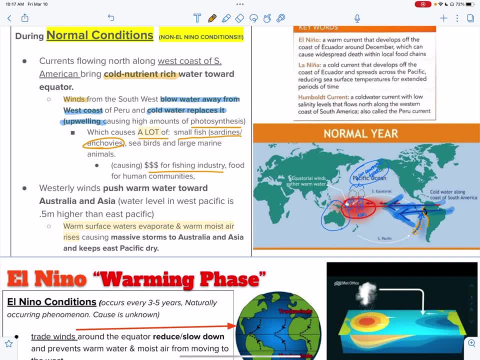 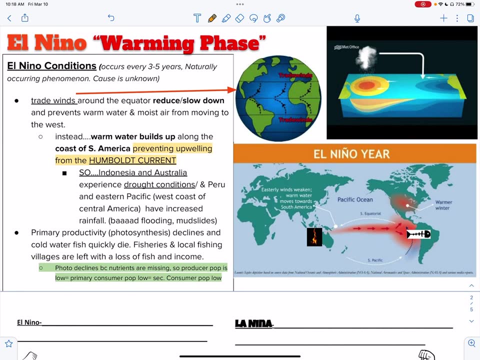 everything that I've just mentioned was a non-El Nino year. okay, and that's pretty much what I just talked about with the precipitation. so during El Nino, your trade winds can completely weaken or they can actually reverse. in this picture you have here, our trade winds have reversed and gone. 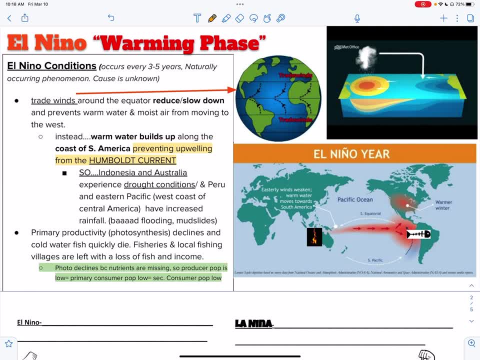 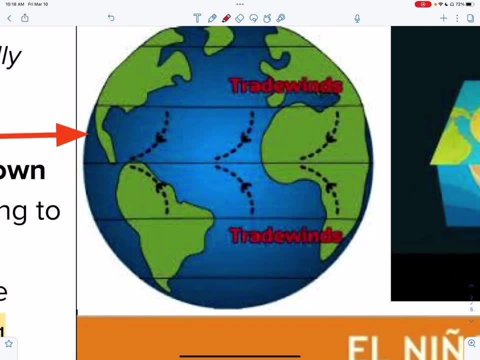 the other direction. um, in our exam answers, though, we're going to talk about them weakening, and so I'll annotate what we're doing in class today. um, below here. so the trade winds. again, trade winds are what blow across the equator. something to recap from earlier this week: notice: this is zero. 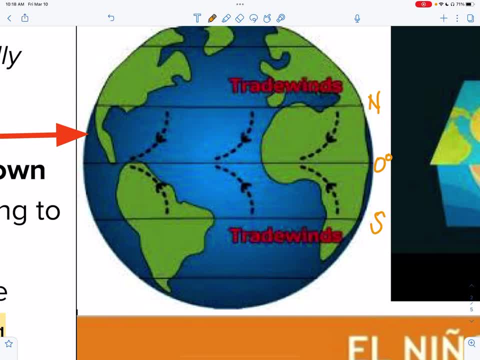 degrees. here's your northern, here's your southern hemisphere. due to the spinning of the earth, Coriolis effect happening so in your northern hemisphere, and granted, that's on, that is land, but in the ocean your water is going to be deflected to the right or clockwise. 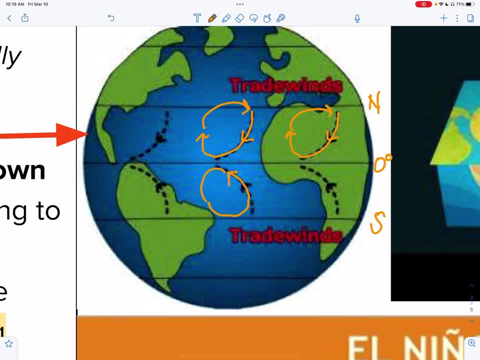 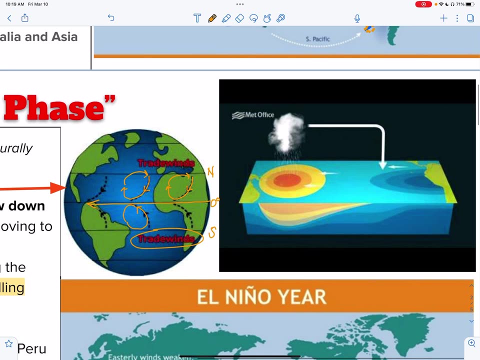 likewise towards the left, or counterclockwise in the southern hemisphere, just to recap earlier this week. but these are your trade winds. they blow across the equator, in the southern hemisphere, low um air which then moves water across the equator. okay, um, ideally, when you guys did your lecture notes, you should have watched. 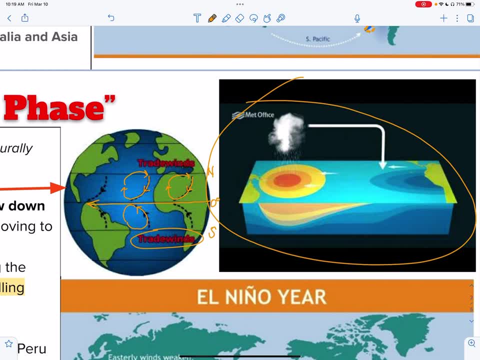 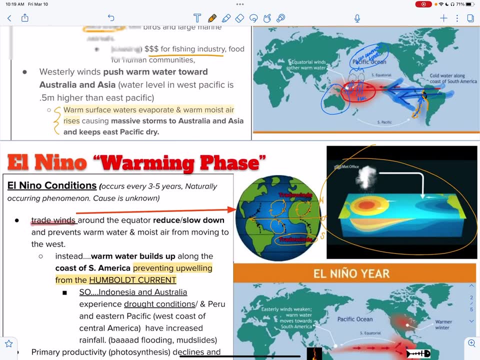 this video. that's what i showed briefly in class today. um, it shows both of these. there's a lot of content in there, some atmospheric talk that won't necessarily pertinent to our syllabus, but it is helpful to see this happening. all right, i'm going quick because my planning is short today. 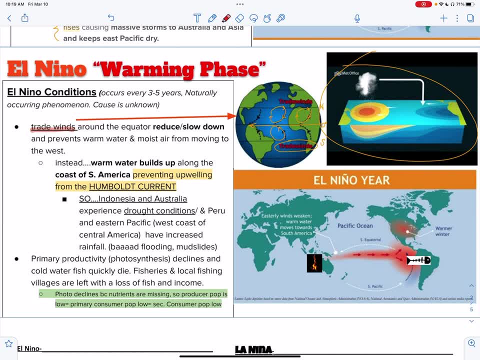 but here we go. um el nino, what we're going to want to start with is that the winds, trade winds that blow around the equator slow down, they weaken. you can mention that they can also reverse, just based on this picture down here. you don't have to. my exam answers always go with trade winds weekend. 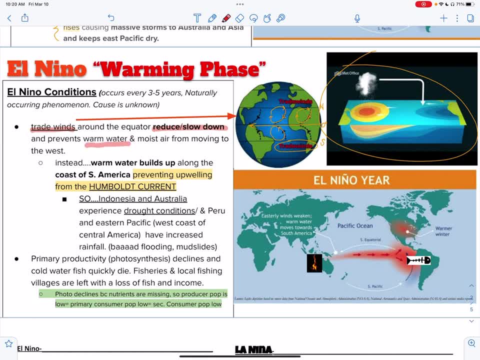 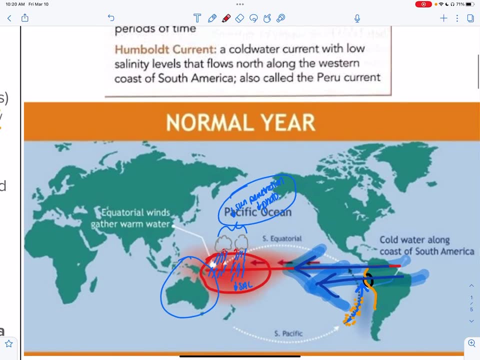 okay, and so this is going to stop the warm water that's piling up at the equator, that warm water from going towards the equator is going to go towards australasia. it's also going to prevent there to be any sort of precipitation like we saw right here in the australasia area. 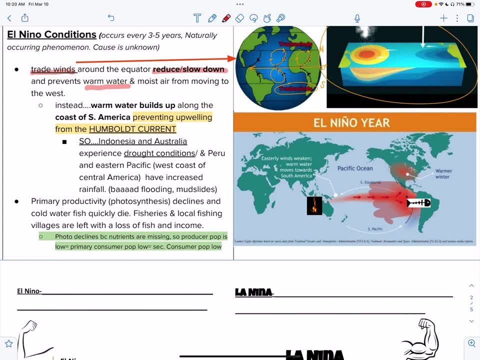 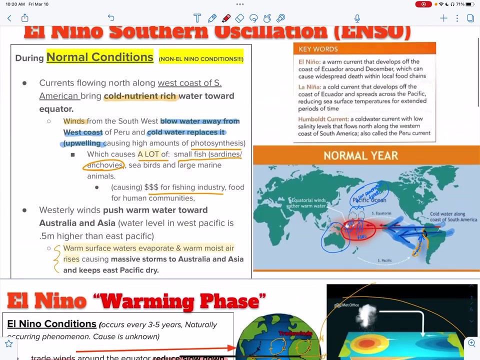 instead, those things are actually going to happen off the coast of peru. so instead, warm water builds up along the coast of south america, the west coast, along where peru is- click with my orange right there. so we're going to start with the cold water current, which is a very common event or extremely weekend. 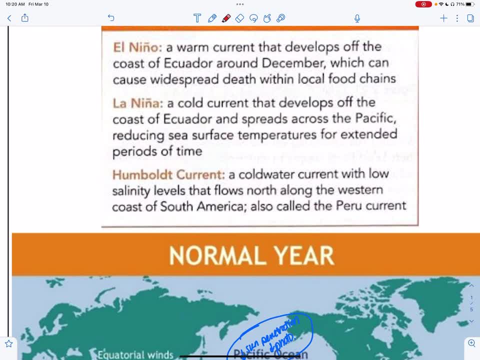 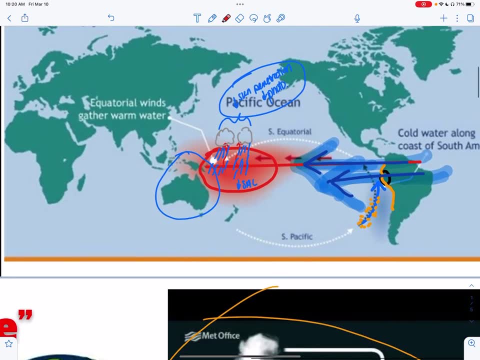 upwelling from that humboldt current, which is one of your vocab words definition right here, a cold water current with low salinity levels that flows north along the western coast of south america. it's also called the peru current um in your exam questions. i really only have ever seen it called the humble. 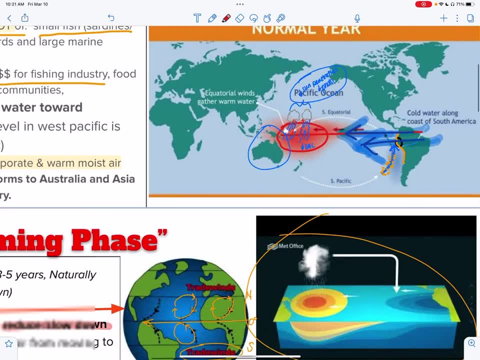 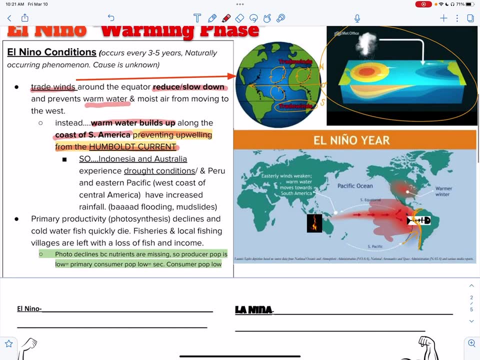 current, but also called the peru current, and if it's upwelling, then we know it's not just bringing up cold water from the ocean support, it's bringing up cold water from the ocean and it's doing it is it is making it so that it can. 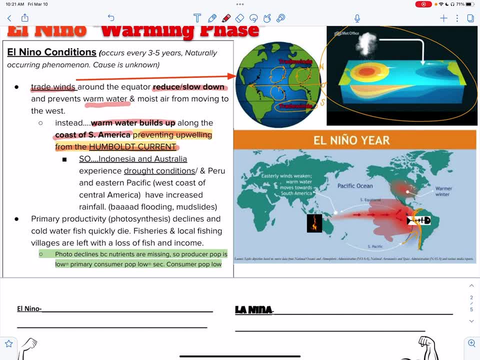 actually be used in the ocean as well. so let's get right into the final part of this and then we just have to remember that. so, for example, when we're going to ask a question whether or not we want to use water flow, we are going to remember to remember that. 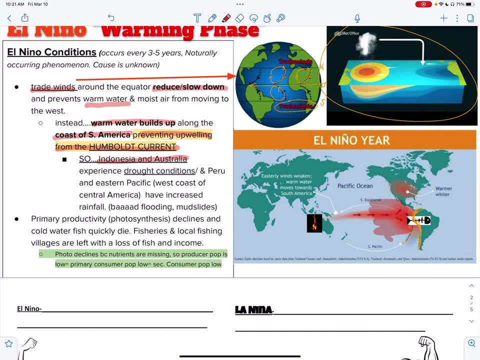 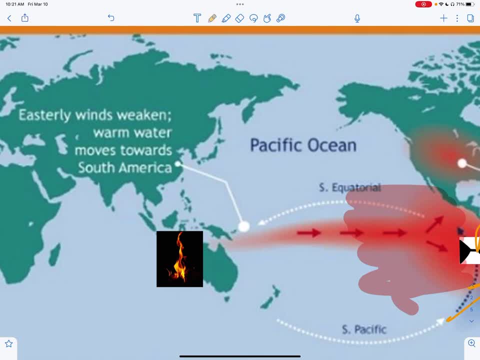 um, we are going to remember where we left off, and what we're going to do is we're going to think about this first, the content of our, our, our, our oceanic water, and then we didn't know, you know, if it was going to be cold. 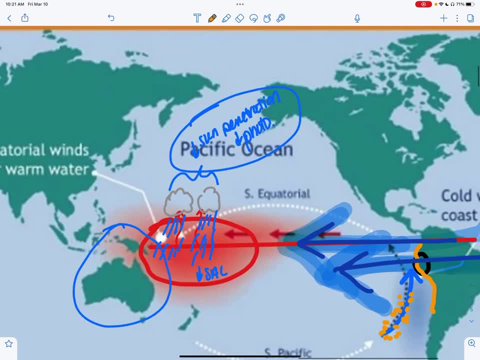 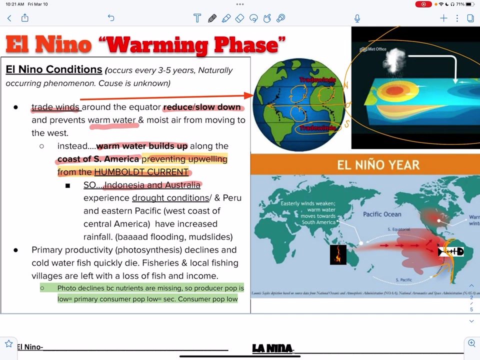 that warm water caused a lot of cloud cover, which is good for precipitation, And so regions over here might be in a drought situation now because they're having a lack of precipitation. there, They'll also have a lot of wildfires, But again, the exam questions don't focus on the Australia-Indonesia area. 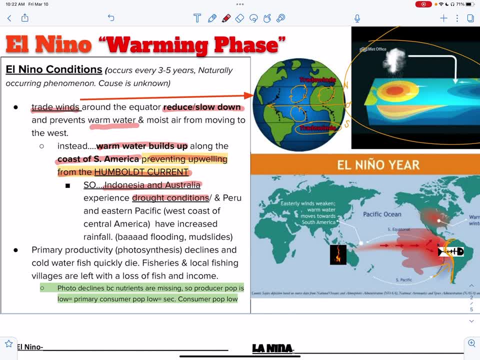 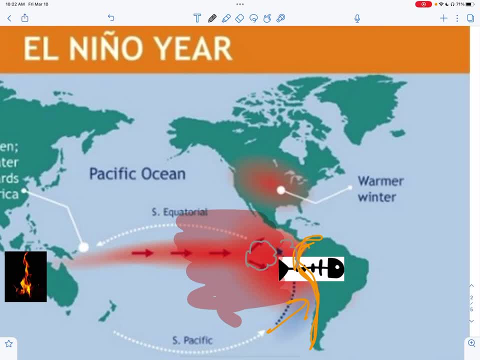 They can have drought conditions. What will happen on the flip side, though? so if we have all of these clouds forming over here due to all that warm water and evaporation- because that water is really warm, what will happen instead over here is a lot of rain, and that could decrease salinity. 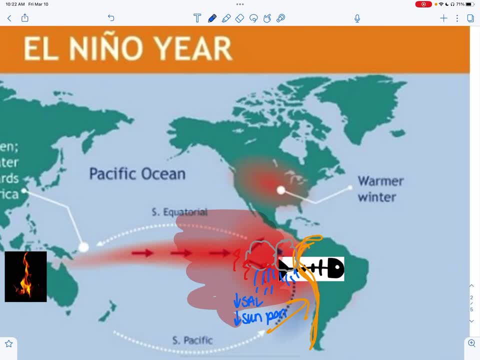 Of course, we're going to decrease the sun penetration from the clouds, And so- Though again, this isn't something that's necessarily tested material, Peru and Argentina, your west coast countries of South America, they're very mountainous, They're built on a subduction zone, essentially. 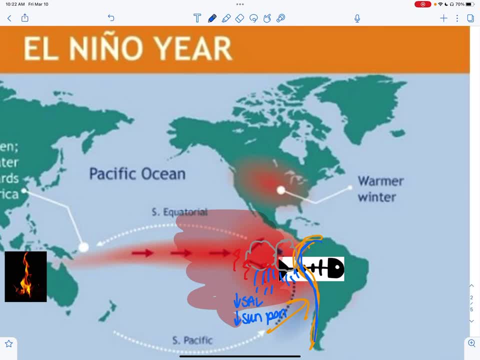 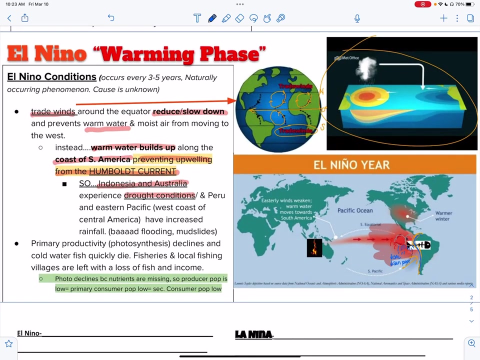 So they have some volcanic action or dormant volcanoes, and they have really high elevation and a lot of high topography. They're going to experience a lot of mudslides, rockfalls, landslides, lots of rain, lots of flooding and not much fish. 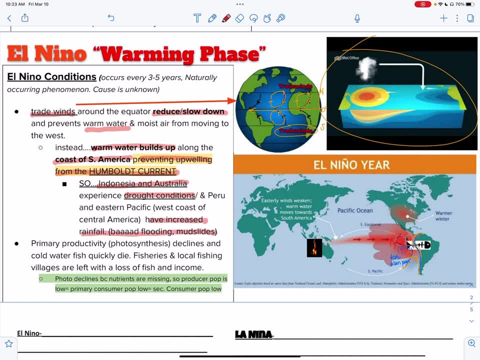 So we have an increase in rainfall, bad flooding, mudslides and that's going to be Peru. Photosynthesis or primary productivity: Productivity definition is the rate of photosynthesis, how fast glucose is being made, But that is going to decline quickly. 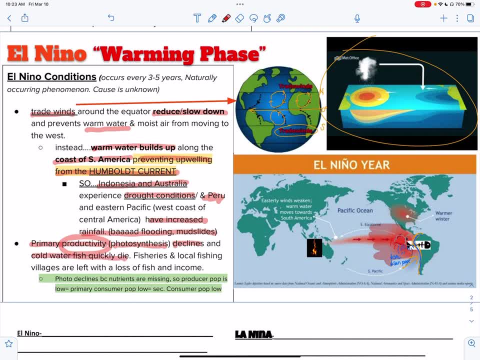 And fish that need to thrive in cold water will also die quickly, because you're going to have a lot of fish that need to thrive in cold water, So you're not having that upwelling. bringing cold water, Productivity goes down again. photosynthesis: 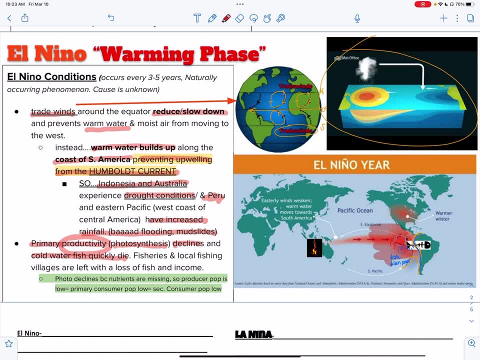 because, again, you're not having the upwelling of nutrients And if you consider them like fertilizers- again not something you would write on a test- that's what feeds your producers, And if your producers are happy, then your primary consumers are happy. 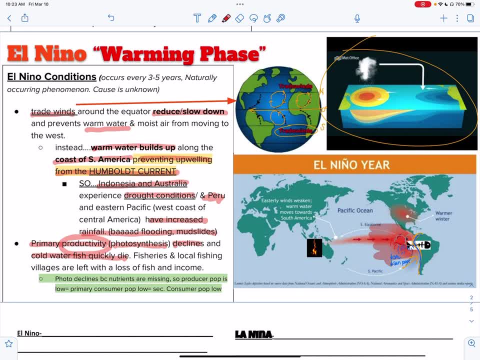 And then secondary consumers, and tertiary and then quaternary, and your food chain as it follows. Animals will migrate down to this area. Obviously, they don't know if it's going to be an El Nino year or not. They can't discuss that with each other. check with the weatherman. 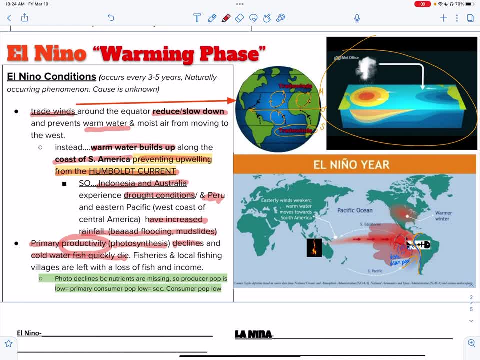 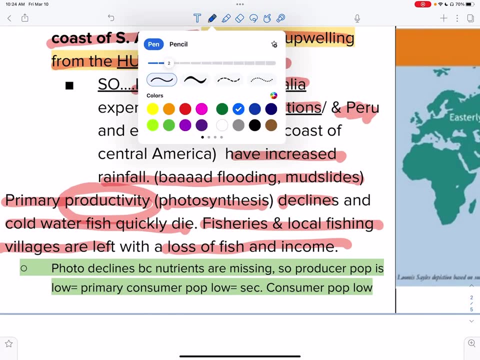 But they will migrate down here and there's going to be no food available. Fisheries- fisheries are what you would call fishing companies, but fisheries and local fishing villages are left with a loss of fish and income. All right, and though it's, this is a very important statement. 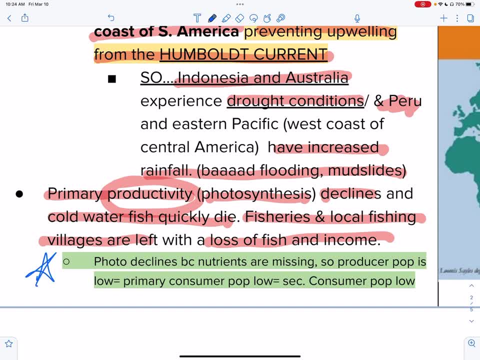 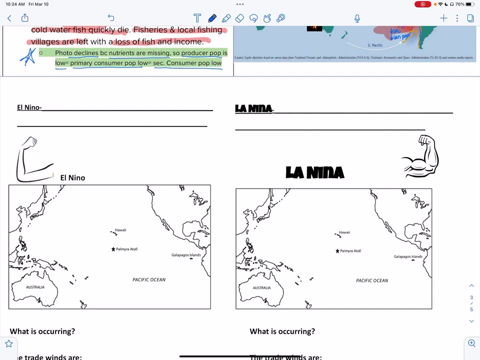 it's, of course, the smallest way to go. Photosynthesis will decline because nutrients are missing. So your producer poisons. Population is low, Primary consumer population is low, Secondary consumer population is low, and so on. All right. What I first talked about was during a normal year. 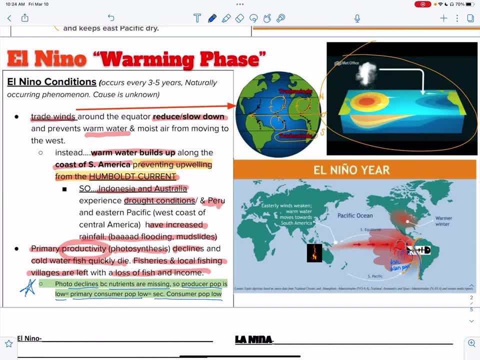 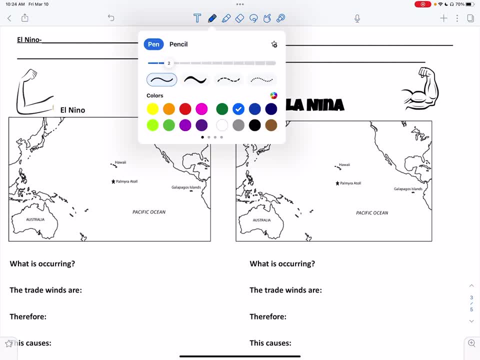 This is during an El Nino year, a warming phase, So when we have the weakening or the complete reversal of trade winds, And so in class we filled this out and you have a blank copy of it on your Google Classroom: El Nino, La Nina, a place for you to put your definition. 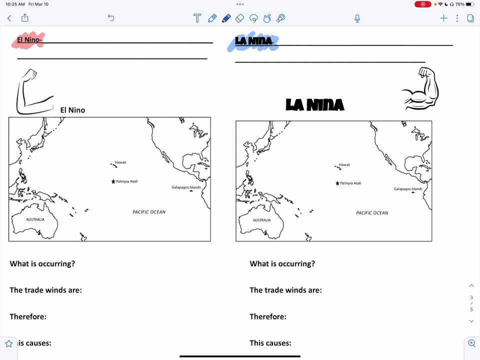 I'm not reversing like gender colors- There is no such thing literally. But El Nino is a warm current that develops causes widespread death in local food chains. La Nina is a cold current that develops off the coast of Ecuador or Peru. 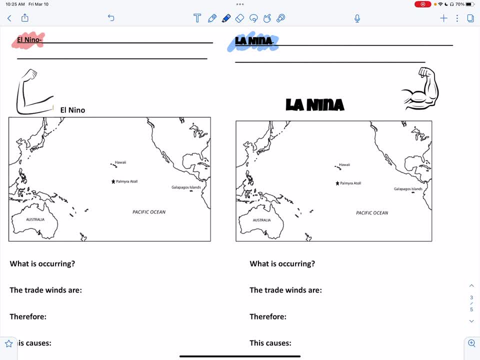 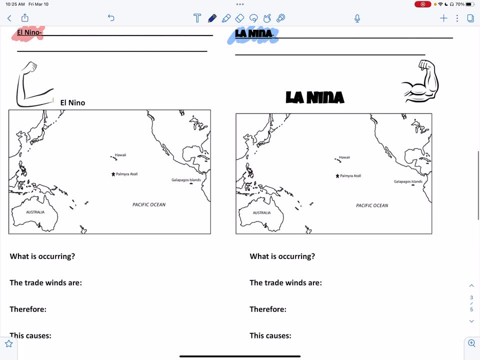 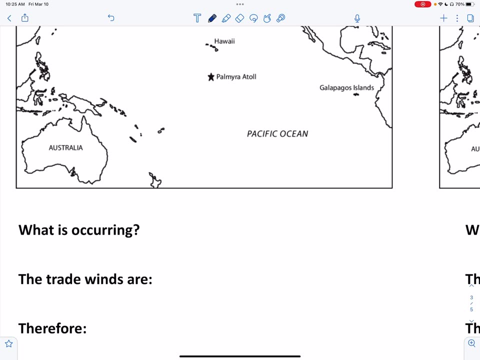 And it will decrease your surface temperatures in the Pacific. All right, So for what's occurring in the El Nino, we're going to have a decrease in the strength of our offshore winds And this is going to keep our solar wind on. 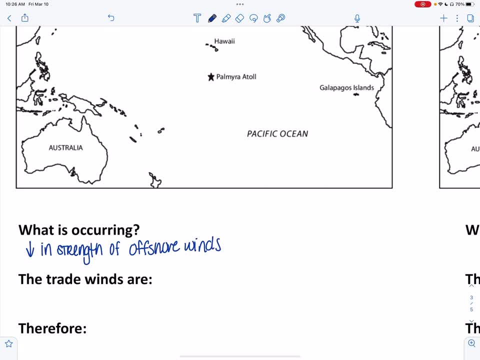 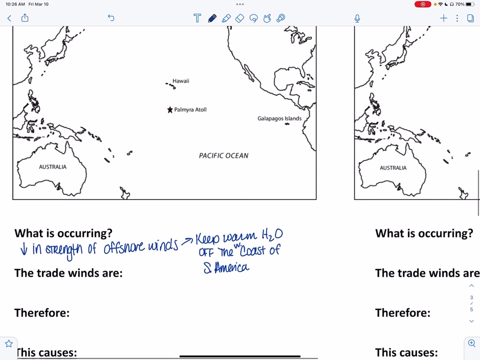 And it's also going to keep energy freely from getting out of the wind. This is that wind we have decades ago. This is it, This is what we're hearing. so far, No wind. We're hearing no. each other heat, warm water, right off the coast of South America, and it's the west coast of South America, our 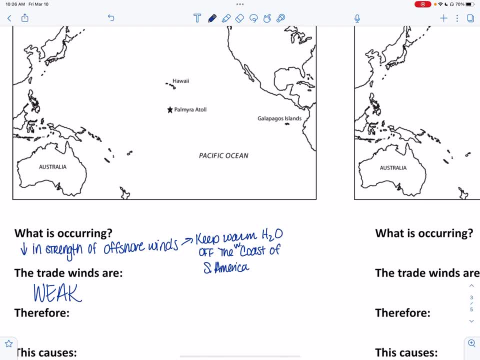 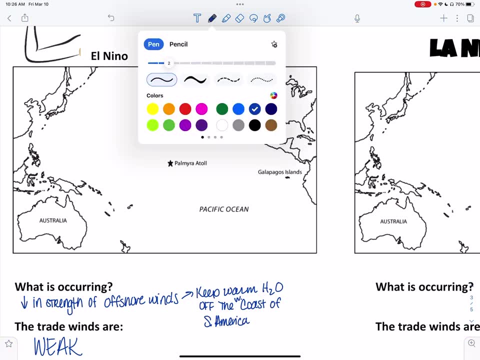 trade winds are weak or completely reversed. but again, just for the simplicity of it, I'm just going to keep it like that, all right. so I'm just going to do an arrow. first, I'll show you the equator. here's about the area of the equator. that'll be my arrow for the. 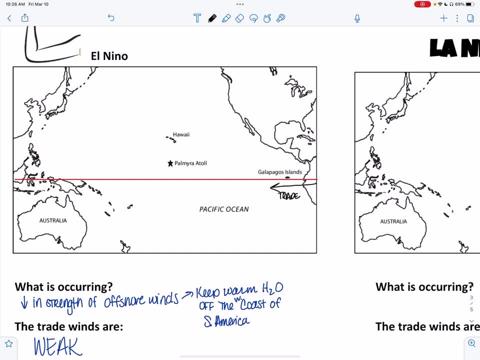 trade wind, nothing grand about it. all right, it's going to keep all this warm water. you're right at the equator, right, zero degrees. it's going to keep all this water piled up over here instead of going with a strong trade wind getting blown over to. 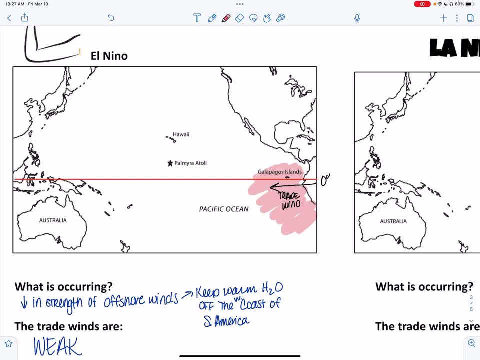 the Australia Asia region, and so a couple, a couple things are going to happen. I'll discuss one at a time. with all that warm water, you can have a lot of evaporation happening, so we're going to have a lot of cloud formation. okay, clouds bring on precipitation. 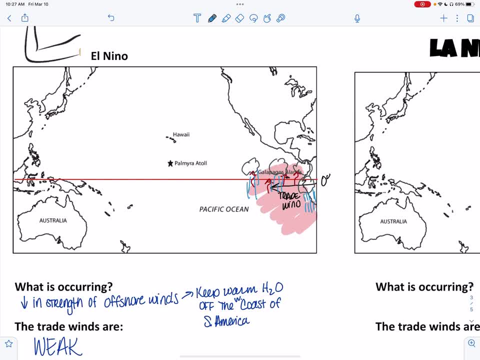 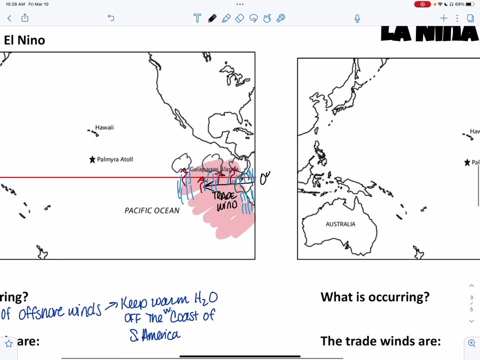 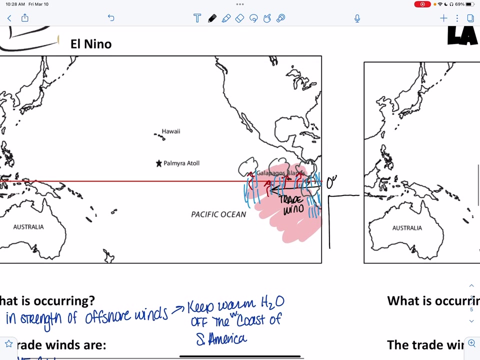 it's going to decrease some salinity, therefore cause the density to change. okay, and off to the side, I'm actually just going to sketch what will be a quick thermocline so we can see how that will change. pause this where you need, of course, consider the sunlight penetration. 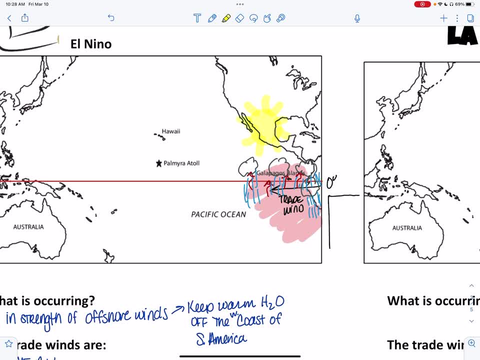 with a lot of clouds, sunlight penetration isn't going to be great, okay. somebody's knocking at my door and if I pause, I'm scared that it's not going to like rerecord, so I'm not going to answer it. that's not going to be good for photosynthesis. 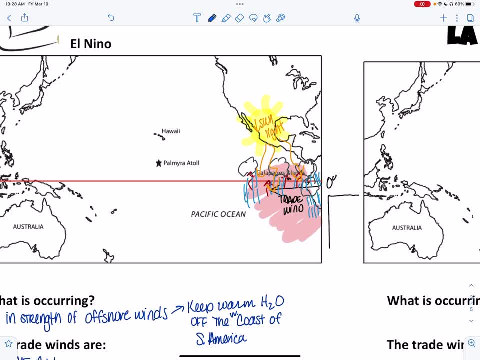 that's sunlight penetration. clouds will bring on a lot of with your storms. rather okay, it's going to be stormy, so you're going to have a lot of waves. they should go the other direction. there we go, you'll have a lot of waves and that's going to stir up your water. 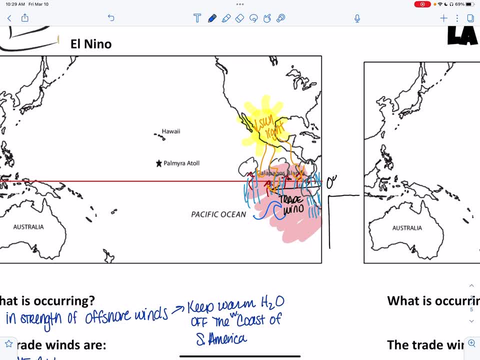 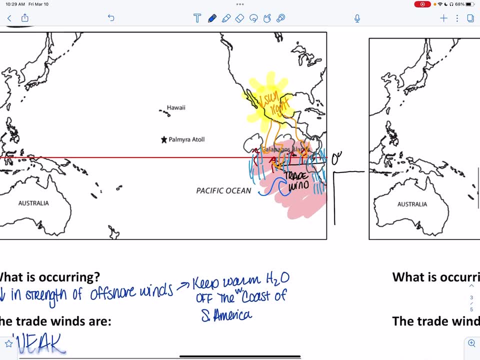 lots of turbidity. so another reason: where sunlight penetration is going to be low, you have the cloud cover and you're going to have a lot of waves stirring up the sediment, stirring up the water. all right, and for any producers that are there, I haven't talked about the nutrients yet. 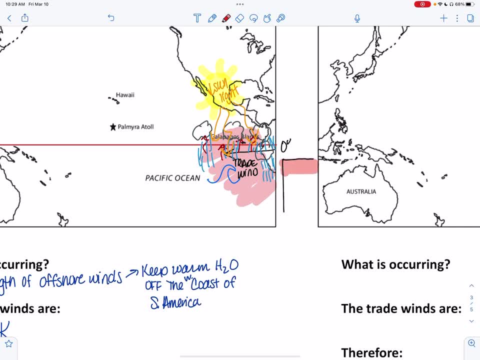 but we have a lot of warm water piled up. a lot of warm water piled up, not just a little bit the surface. there is a surplus. I can't answer right now, I'm sorry. I don't trust pausing it temp and obviously we have depth here in meters. 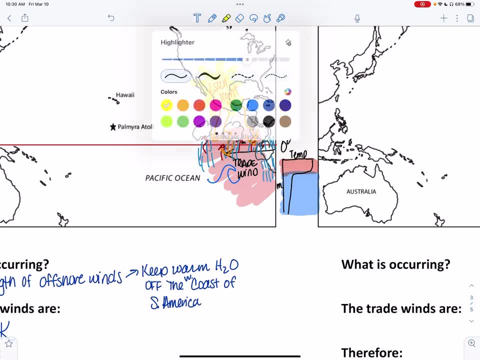 why does this matter? so the thermocline keeps really low dense water at the surface and when you have little phytoplankton they need to be at the surface. they don't have arms, tails or legs to swim up towards the surface to be in sunlight. 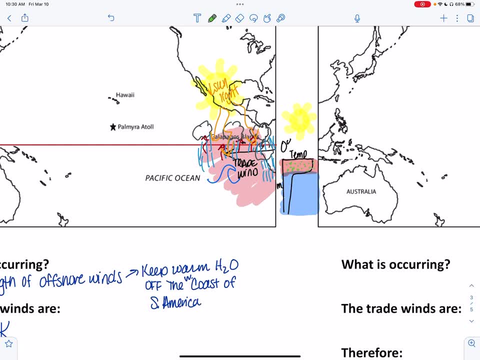 so they're stuck at like the mercy of your top floating low density layer of water, because it's very warm, so you're going to have a lot of water, and where a thermocline may have previously have been, maybe here. right, that would keep them up higher in your water column. 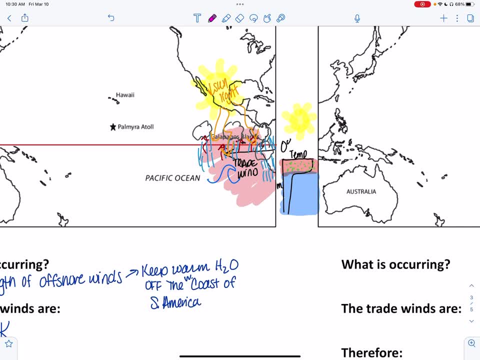 well, now you have so much warm water piled up that you have a lot of warm water for the surface layer and that just causes you to have a deeper area of warm water if your sunlight can only penetrate so far. right in the open ocean it's about 150-200 meters. 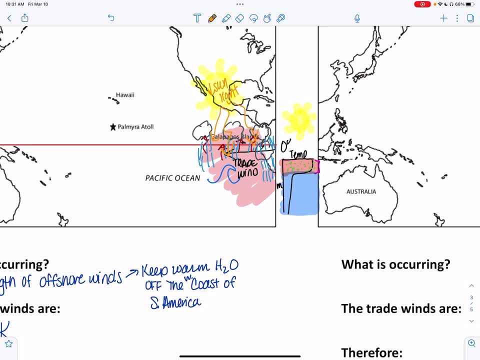 but on the coast it's about 50 meters because of waves and wind. what if the sunlight's only going this far? with all that warm water piled up, you have a thermocline that's much deeper. and those producers, your phytoplankton, the ones down here, 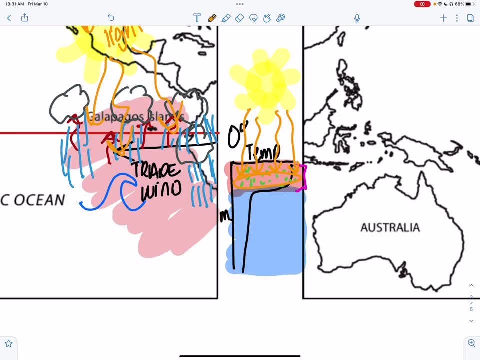 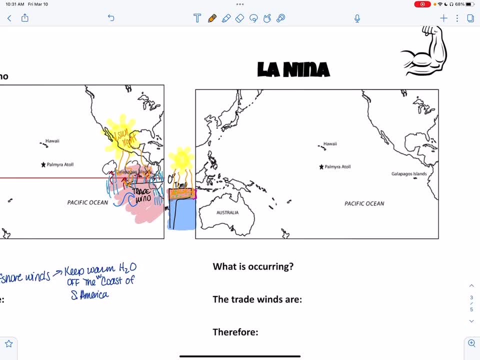 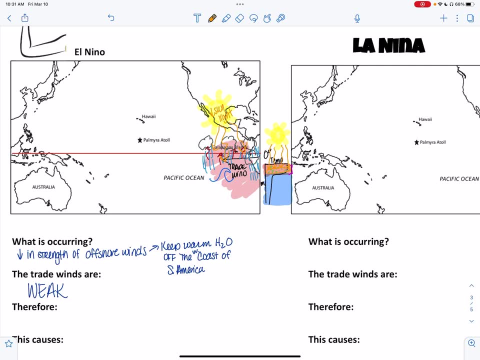 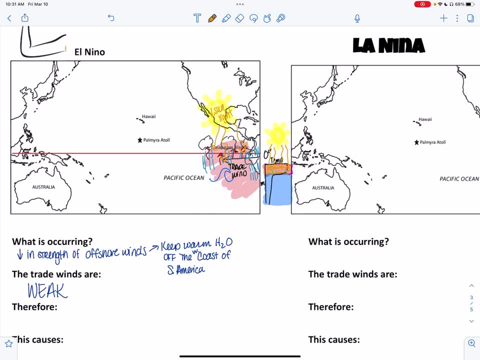 the cloud cover from the increase in evaporation. so therefore you're going to have a precipitation wind causing waves, excess turbidity. none of that's great, but the the main thing that we need to consider is what's going to happen to the humboldt current. 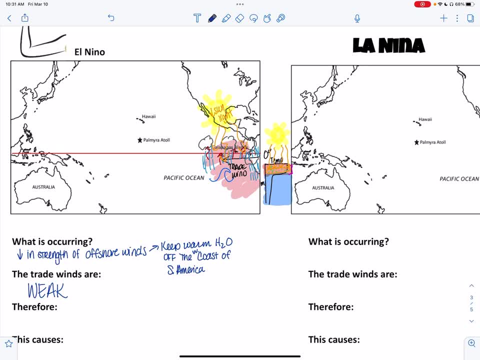 so we know that upwelling is going to happen. so we know that upwelling is going to happen when you have offshore winds, and we just showed that our offshore winds are much weaker during el nino- the trade winds that blow across. they're much weaker. 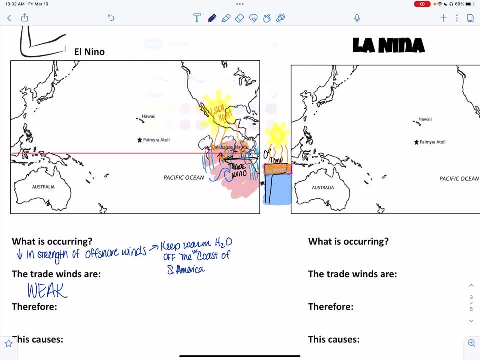 so if there's upwelling, it's also going to be weak, tiny arrow. my arrows will definitely be different between the two pictures: humboldt, current, all right and again, the reason why i put videos and notes is just to support you with things that i can't show you. 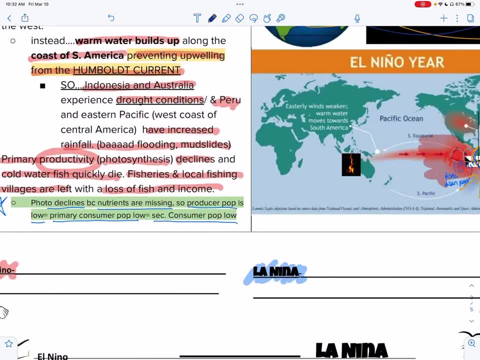 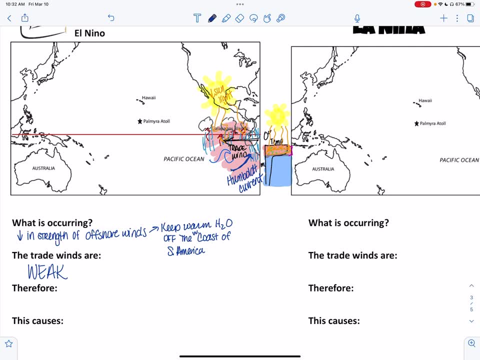 so this video is doing the same thing, essentially, with some more terms that you won't necessarily need for your exam. um, that i am. tree. winds are weak, so let's finish out what we're putting for our exam answer. therefore, we're going to have low upwelling. 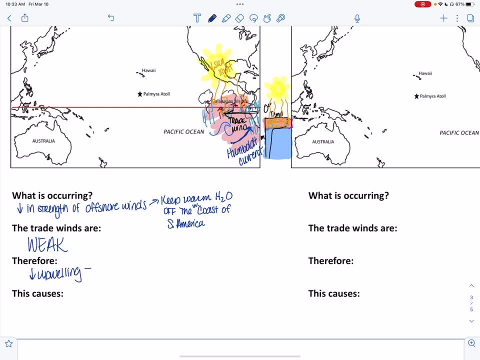 we're going to have low upwelling, which causes low amount of nutrients coming up again. these aren't nutrients for animals, these are nutrients for producers. nutrients like nitrogen, phosphorus, things that cause algal blooms in our indian river lagoon when we have a surplus of them going in. um sulfurs, potassium, calcium, magnesium. when you plant the magnesium to synthesize chlorophyll, so they can absorb sunlight, nitrogen, phosphorus. those things are needed so they can make um amino acids which make proteins enzymes. they also need to make nucleic acids like, so you can synthesize dna or rna. 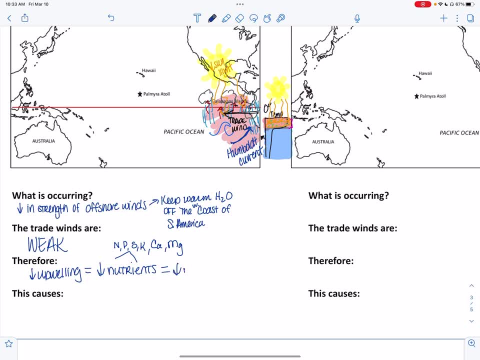 so if you have a low amount of nutrients, we're going to have a low producer population. if you have a low producer population, consider your trophic levels. trophic level one, two, three, four producer is always on the bottom, no matter what. here's your primary consumer. 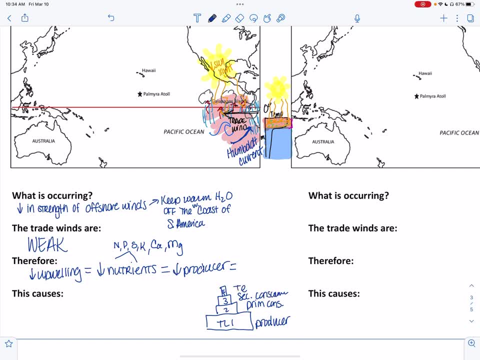 secondary consumer, tertiary consumer and so on. if the producer population is low, what are the primary consumers going to eat? they're also going to be low. everybody suffers, including the fishermen. so, low producer population, we're in a low consumer population. the biggest fly see my students do is this: link right here. 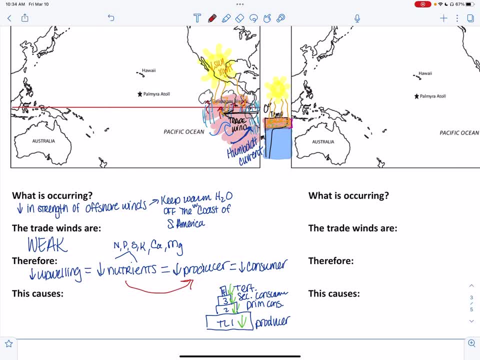 between nutrients and producers, students, all the time will go. there's low upwelling, so a low amount of nutrients, so your fish are going to die. no, no, no, you can't jump to the consumer. we don't feed our fish these things. we don't feed them fertilizer from the garage. we don't. 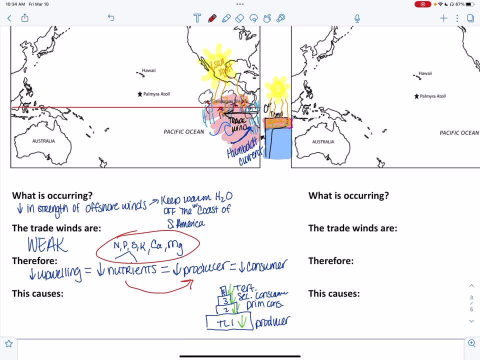 feed them rocks. we don't feed them soil. that's not what we do. consumers, including humans, we can't eat that. all right. and so what will this? what will happen with this? we're going to have a low amount of money for fishermen, low biodiversity, so a variety of species that are in an area and their own like. 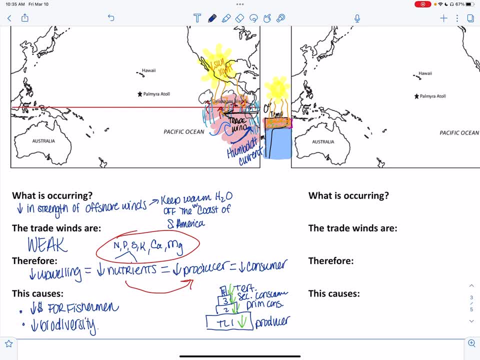 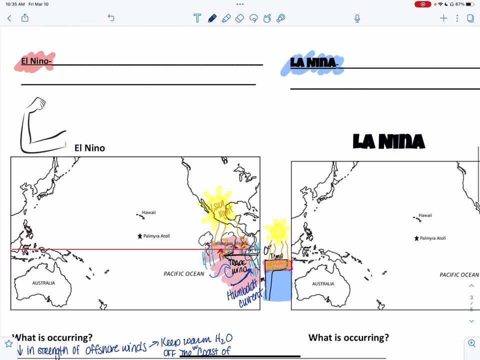 genetic diversity. there will also be low, lots of storms, lots of rainfall. our questions primarily orient themselves towards the lack of upwelling, therefore a decrease in your producers and consumers, and then what that's going to do for fishermen, and we'll see that on the practice exam questions. and so if you look at the 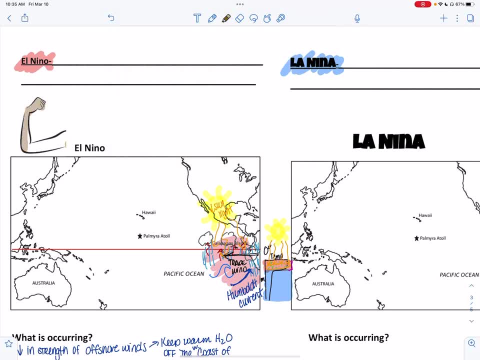 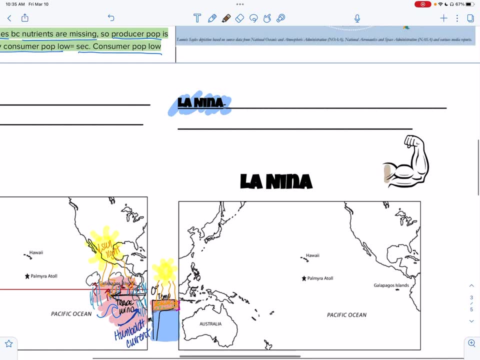 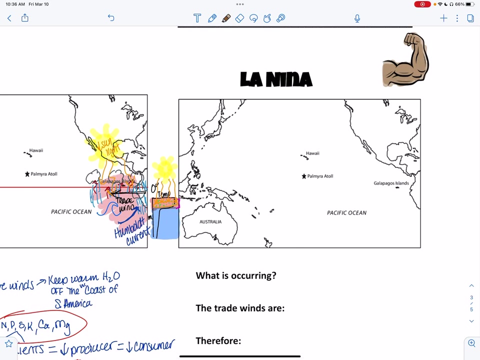 little images i put on there. you're just your el nino, weak, tiny little arm. but la nina, she's strong. look at that arm. good for her, la nina, she's very strong. this is the exact opposite of what's going to happen now. definition: here is the. 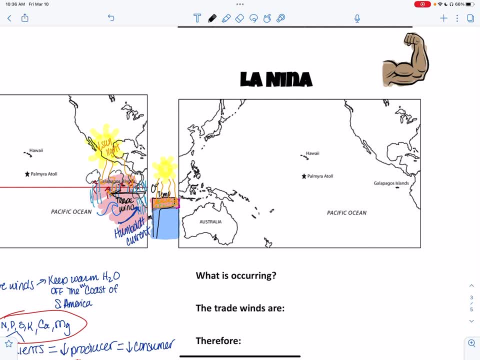 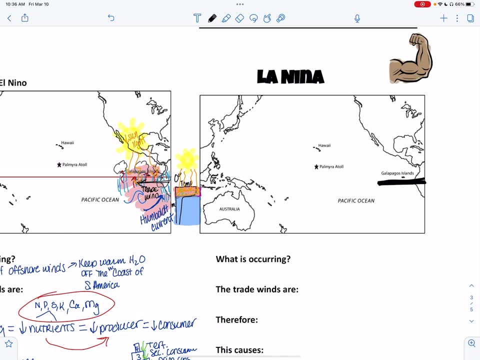 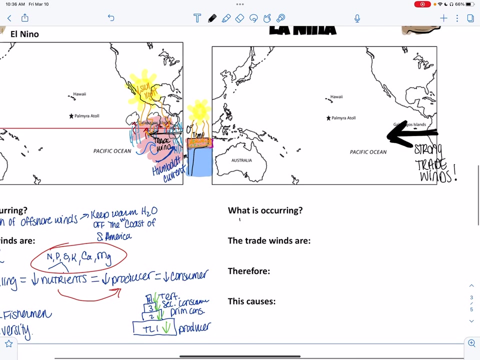 cold current that develops off the coast of ecuador. check this out. so here is my little tiny trade wind arrow: much stronger trade winds, much stronger, strong trade winds. and so what's occurring here? we have an increase in the strength- that's weird- of offshore winds. 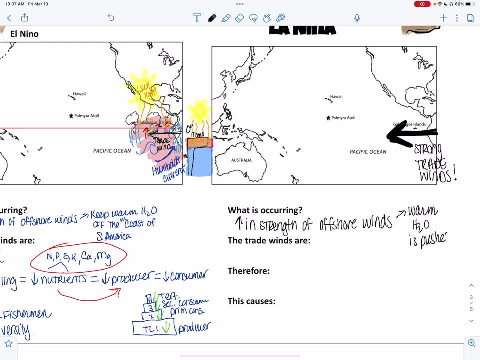 warm water is pushed away toward australasia from the south american coast and the west side of the west coast of it, and so for pushing all that warm water away. this is why it causes cooler temperatures in the pacific, so we're going to have a large pile of cooler water here. 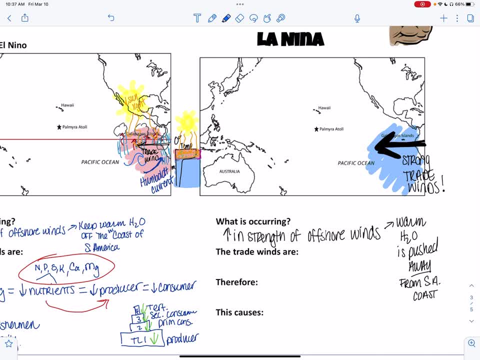 thermal klein will be much higher up. we're not gonna have all these clouds so lacking. people observe color and qu? слова. let's go over not going to have the clouds here, because we're not going to have an excess of warm water with a lot of evaporation and then precipitation, but what we will have is a very strong current a. 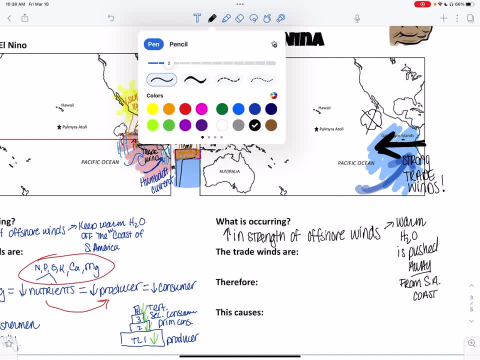 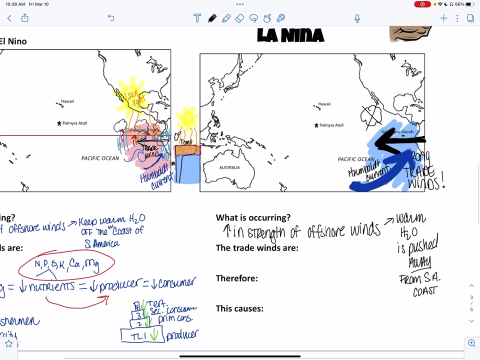 very strong, humble current moving up. i think on your notepaper the arrow size is is a good visual. if the current is very strong, that's upwelling lots of nutrients, producers will be happy, primary consumers will be happy, fishermen will be happy. everybody wins. the trade winds are strong. 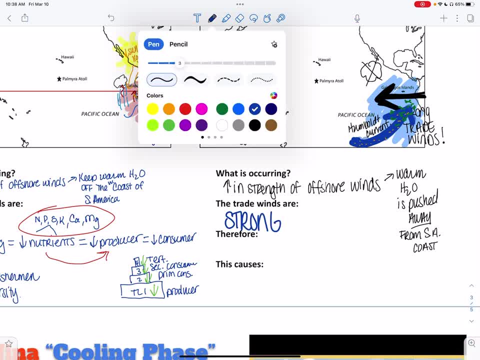 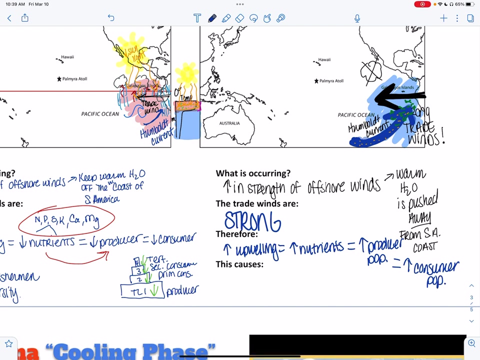 therefore, we're going to have an increase in upwelling. cause an increase in nutrients again. these nutrients are for producers, not fish. cause an increase in producer population, which has an increase in all of your consumer population, so this will cause much more money for fishermen and fisheries. 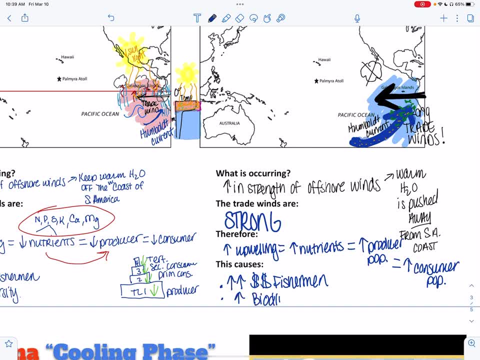 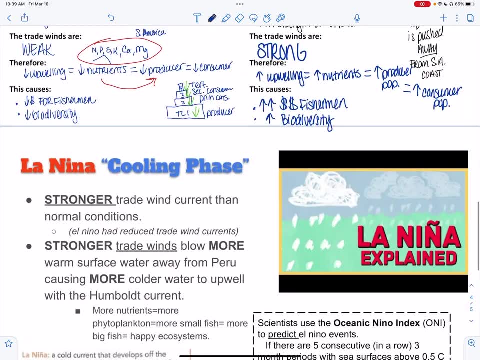 and we're going to have an increase in biodiversity of organisms there. so it's all about the trade winds and what's happening to that humble current. in your notes you should have had that the strongest airwise current is not going to come out of the water.